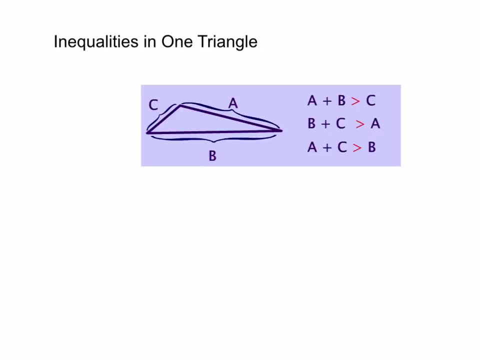 So c plus a must be bigger than b. Now here's how it plays out with some numbers. Suppose that you have three sides. Suppose that you have three sides and you're wondering whether they can form a triangle. Suppose you have the lengths 3,, 4, and 5.. 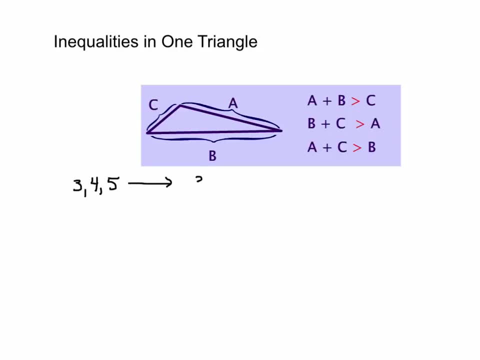 Well, to check and see whether they can form a triangle, take the two shortest lengths and make sure they add up to more than the third length, And in this case we have a triangle. By contrast, suppose we have 13,, 3, and 5.. 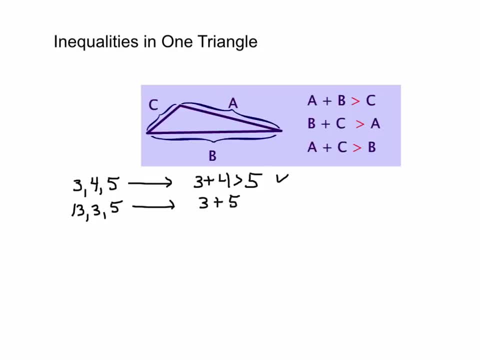 In this case, if we add up the two shortest lengths, 3 plus 5, we get something that's less than 13.. So therefore we don't form a triangle. You can even use a variable here. Suppose that two of our lengths are 13, and x and 7.. 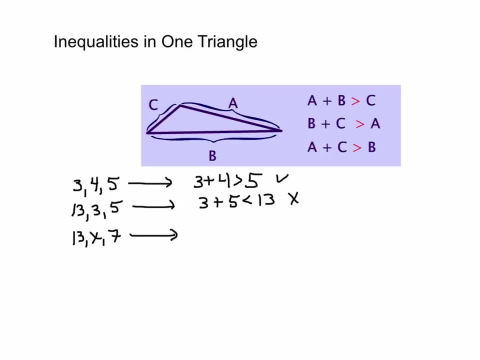 We could then figure out what possible x's will make a triangle, And to do that you want to subtract the two sides and add the two sides and sandwich x in between. So in this case it looks like the third side could be any value greater than 6, and less than 20.. 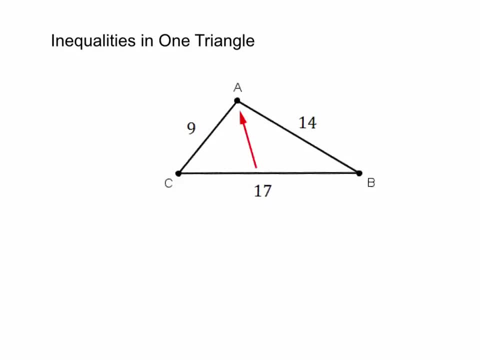 The other key inequality in any one triangle is that the largest side- for example 17 here- is opposite the largest angle. The smallest side is opposite the smallest angle and the intermediate side is opposite the intermediate angle. So if we were to write these angles in ascending order of size, the smallest angle would be angle B. 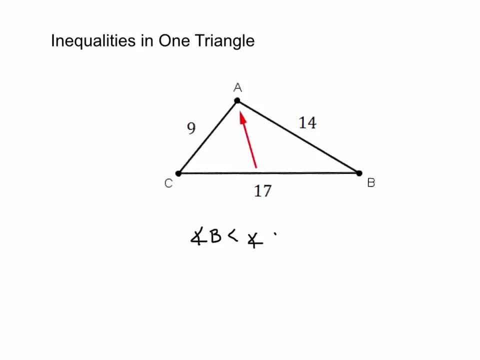 and that's less than the intermediate angle, which is angle C, Which is less than the largest angle, which is angle A. So let's see if we can actually justify this with a proof. So in this diagram we're given that BC is longer than AB. 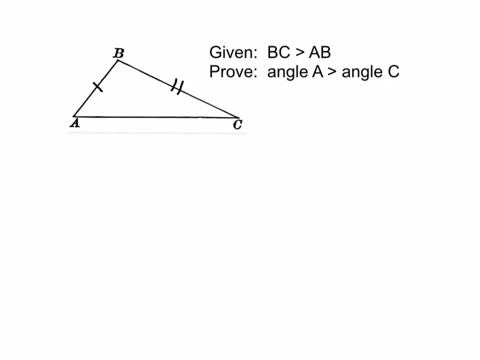 And we're going to try to show that angle A is bigger than angle C And to do that, let's add one more segment to the picture. I'm going to draw a segment from B down to this side. I'll call that intersection point D.